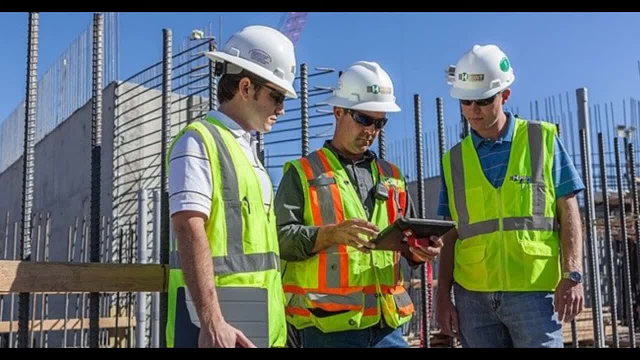 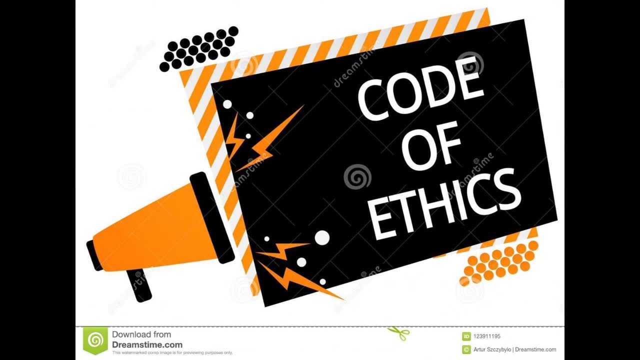 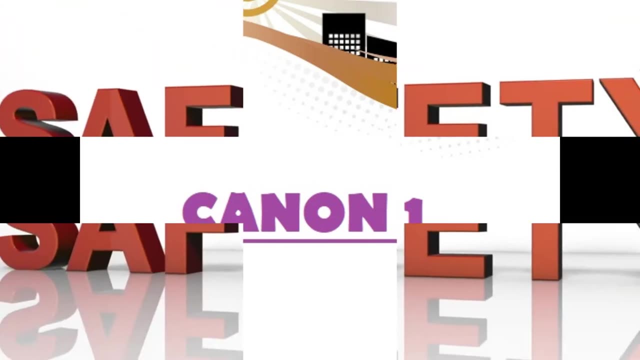 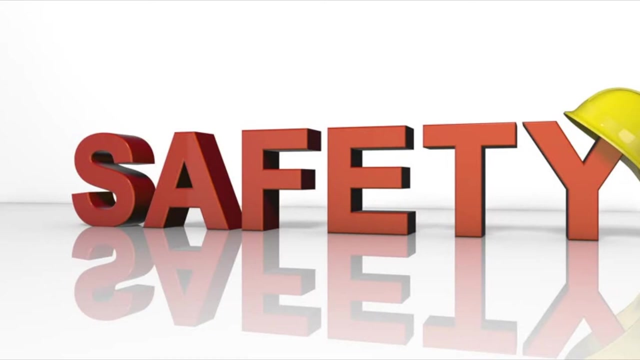 the benefit of the public. professionals are held to a higher standard than the general public in the code of ethics provides the guidelines and standards that the professional engineer must follow to satisfy that commitment. the canon one states that civil engineers shall hold paramount the safety, health and welfare of the public and shall strive to comply with the principles of sustainable. 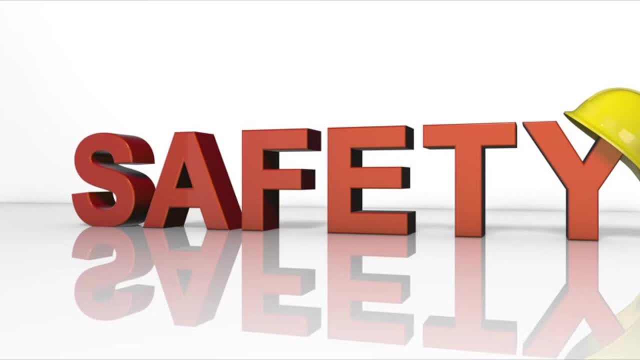 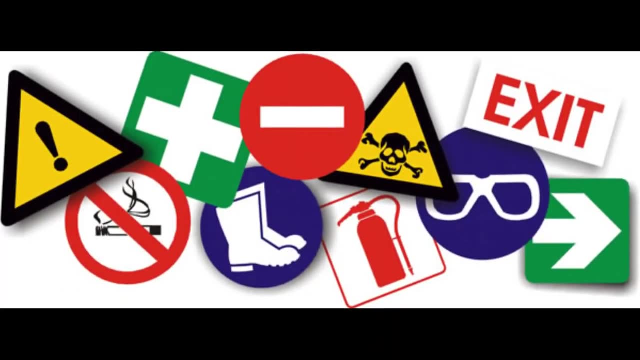 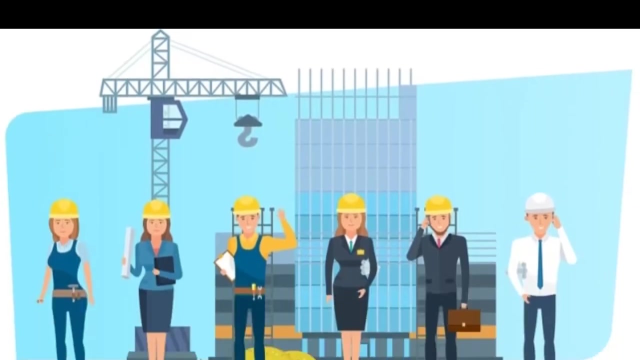 development in the performance of their professional duties. so the general public, depending upon engineering judgments approved design documents, only when it is saved, whose professional judgment is overruled or someone may be is in violation in this can run. they may report to the proper authorities because, as we know, life safety in health and welfare of the general is the 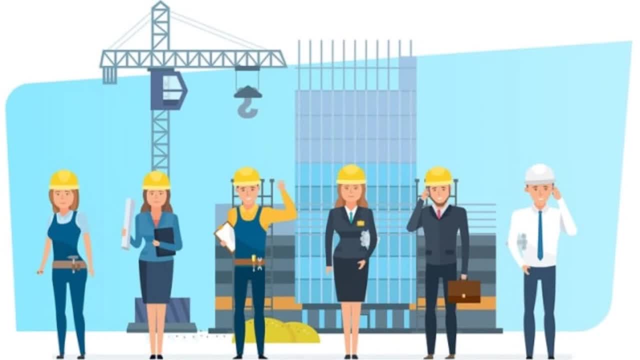 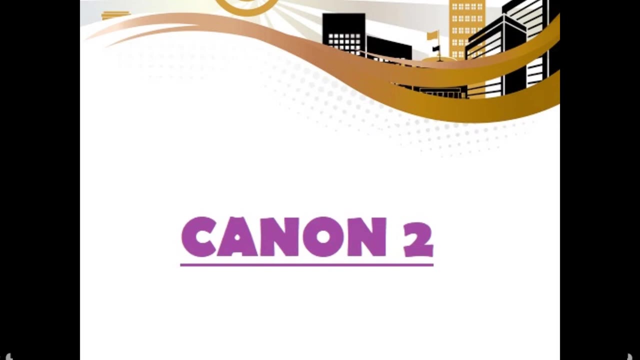 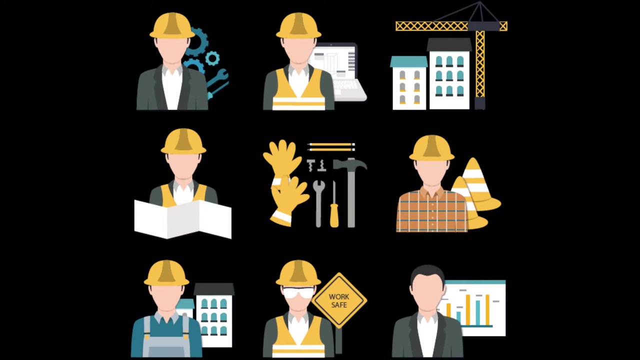 most important of all. so the civil engineers should be committed to improving the engineering by adherence to the principles of sustainable development, so as to enhance the quality of life of the general public. Canon 2 states that civil engineers shall perform services only in areas of their competence. 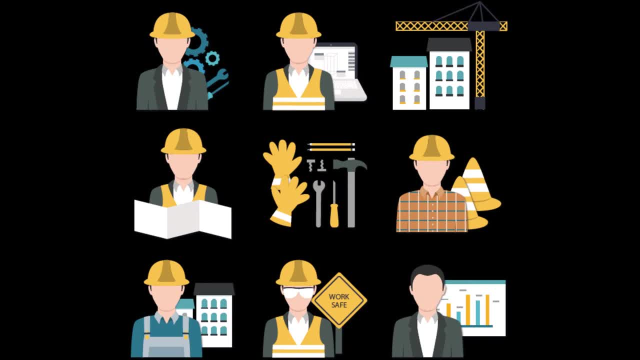 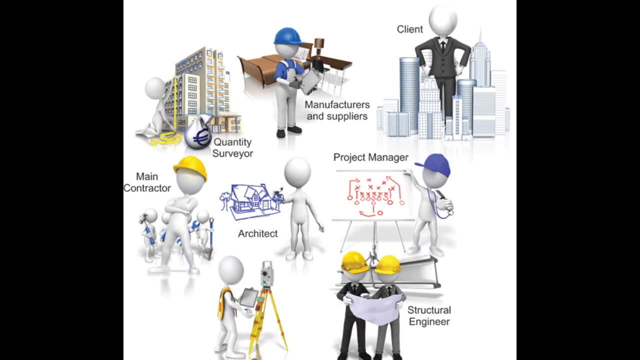 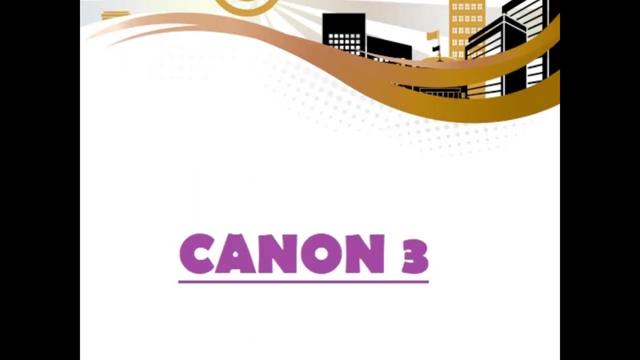 So do not accept engineering assignments when you are not qualified. The education or experience and technical field of engineering is very important. Do not affect signatures which they lack competence. Do not use specialty title without PICE accreditation. The Canon 3 states that civil engineers shall issue public statements only in an objective way. 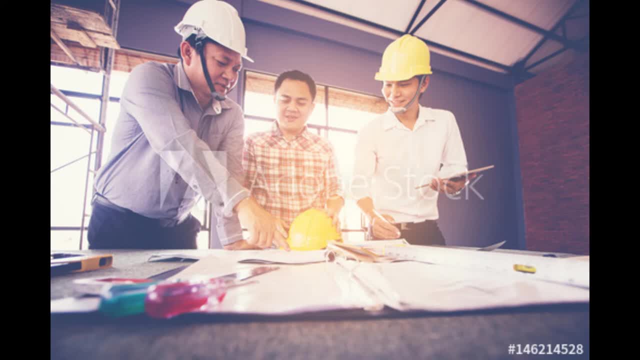 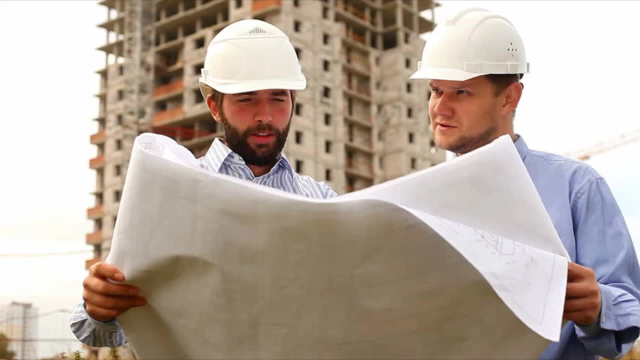 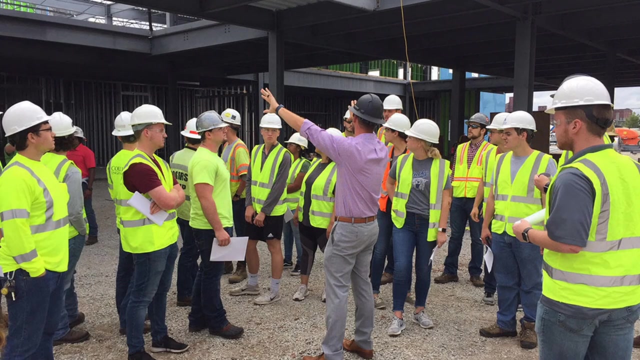 So it shall be objective and truthful in professional reports, statements and testimony. No to criticism or arguments on civil engineering matters. So civil engineers shall be dignified and modest in explaining their work and merit and will avoid any act tending to promote their own interests. 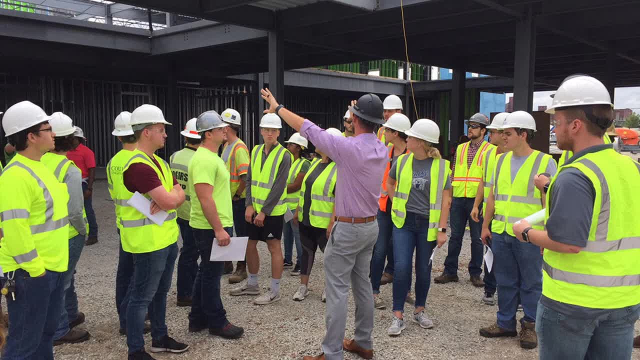 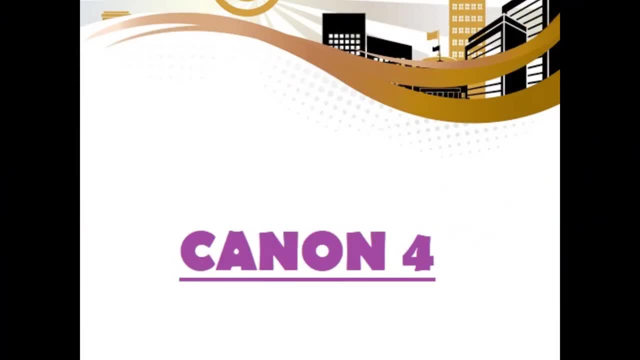 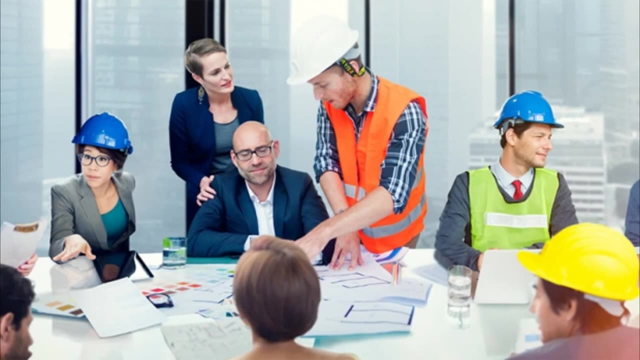 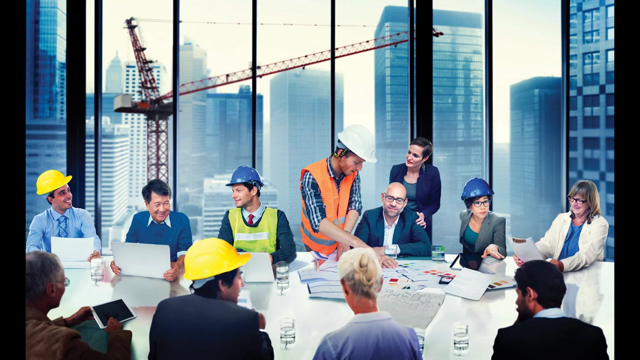 at the expense of the integrity of their work, Honor and dignity of the civil engineering profession and all related professions. The Canon 4 states that civil engineers shall act in professional matters for each employer or client as faithful agents or trustees and shall avoid conflicts of interest. 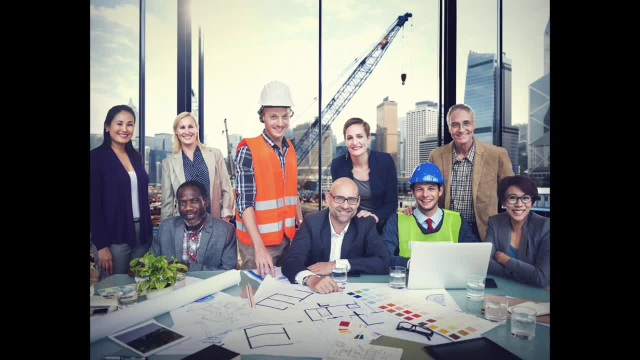 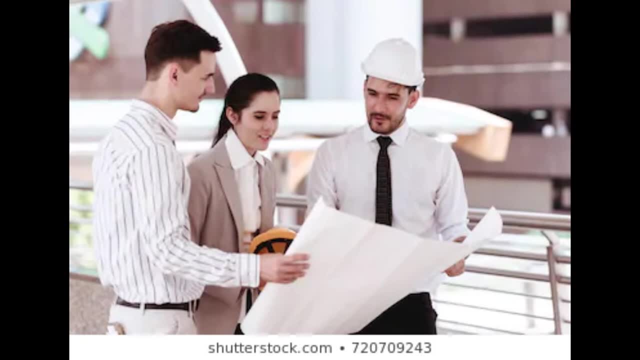 So this Canon 4 says that you should avoid all conflicts or interests with employers or clients. You should not accept compensation from more than one party on the same project. They should advise their clients or employers when project will not be successful or if it will fail. 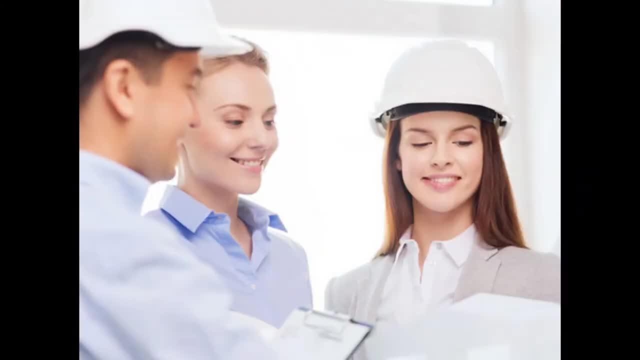 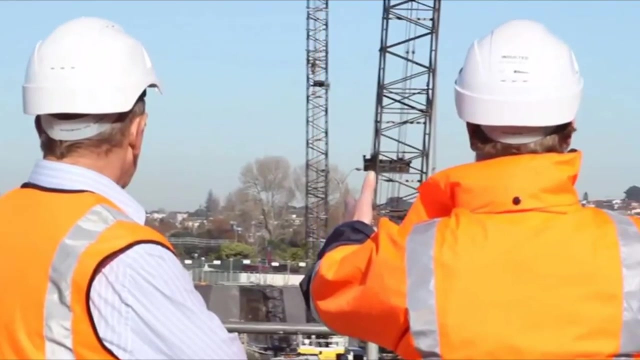 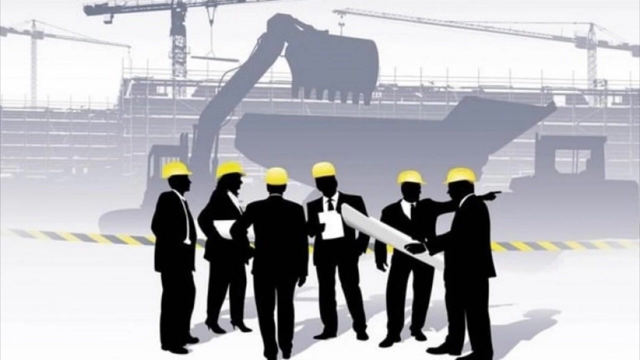 So the civil engineers shall not accept professional employment outside of their regular work or interests without the knowledge of their employers. The Canon 5 states that civil engineers shall build their professional reputation on the merit of their services and shall not compete unfairly with others. So when you are a civil engineer, 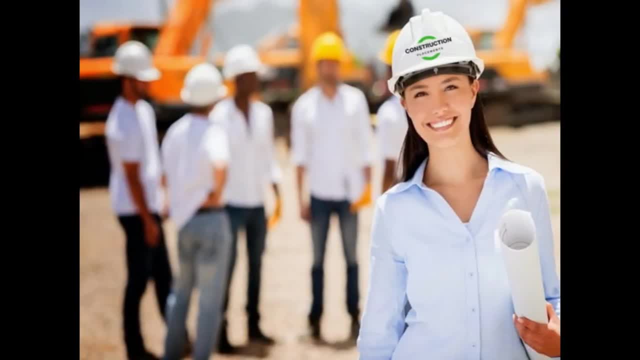 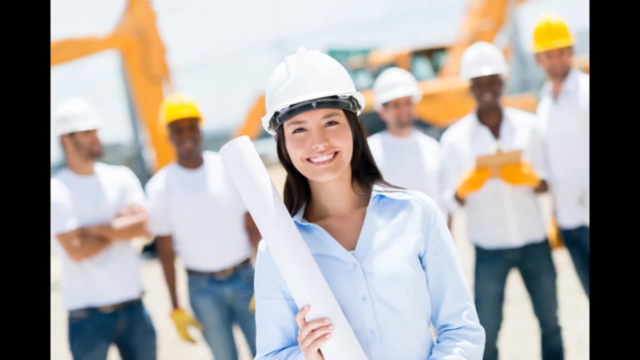 you should not maliciously or falsely, directly or indirectly ensure the professional reputation, prospects, practice or employment of another engineer or indiscriminately criticize another's work, because it is not good. As we all know, we have our own designs. Everyone is different. 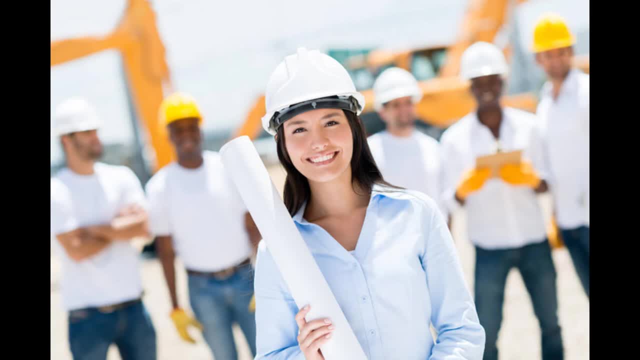 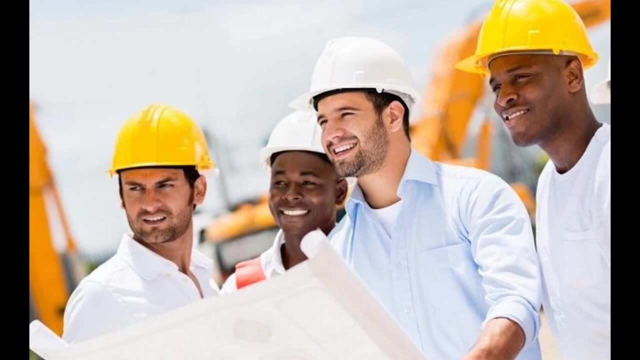 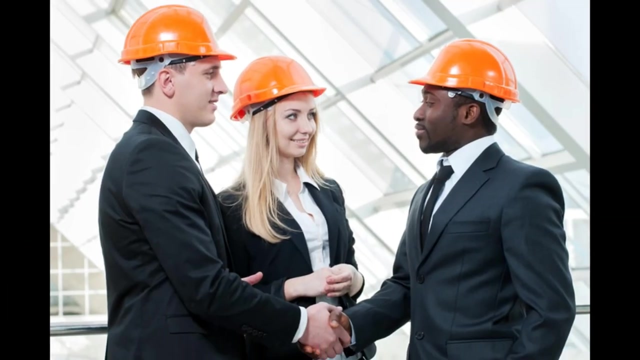 So you could not indiscriminate anyone's work. So you should not B Equipment. I mean you should not use equipment, supplies, laboratory or office facilities of their employers to carry on outside private practice without the consent of their employers. The number 6 Canon states that civil engineers shall act in such a manners as to uphold and enhance. 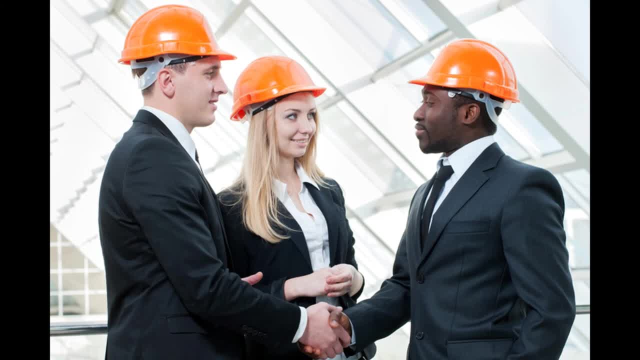 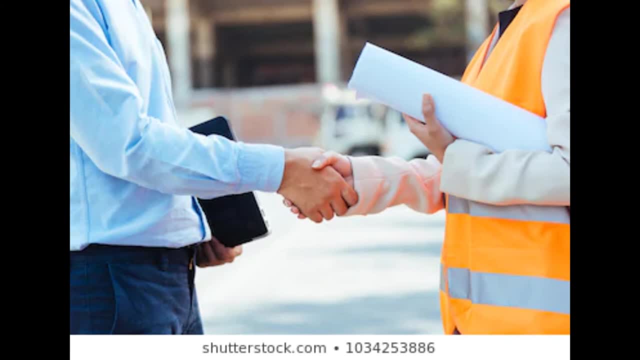 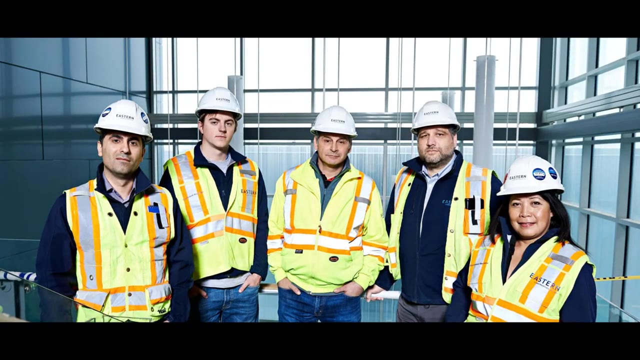 the honor, integrity and dignity of the civil engineering profession. So if the civil engineers shall not knowingly act in a manner which will be derogatory to the honor, integrity or dignity of the civil engineering profession, or knowingly engage in business or professional practices of a fraudulent or dishonest or unethical nature, 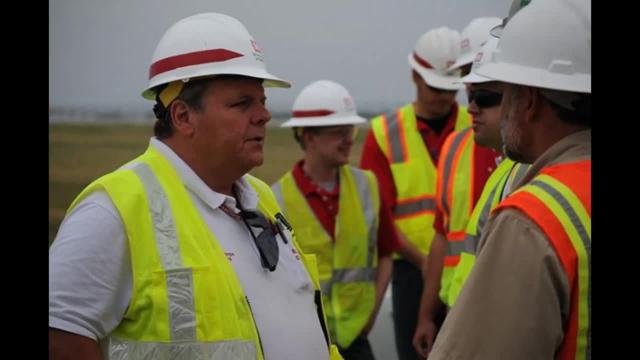 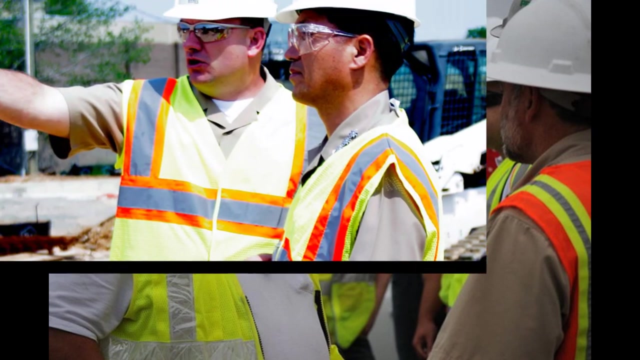 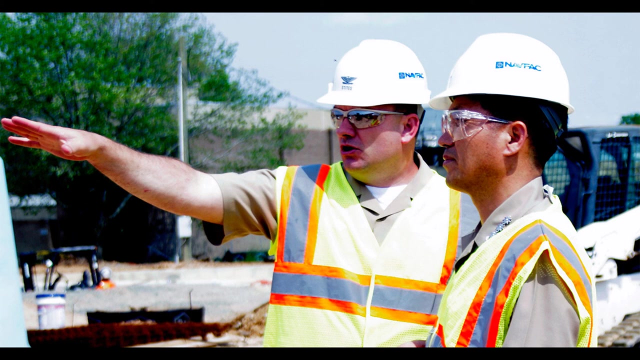 Canon 7 states that civil engineers shall continue their professional development throughout their careers and shall provide opportunities for the professional development of those civil engineers under their supervision. So the civil engineers should keep current in their specialty fields by engaging in professional practice, participating in continuing education courses, something like that. 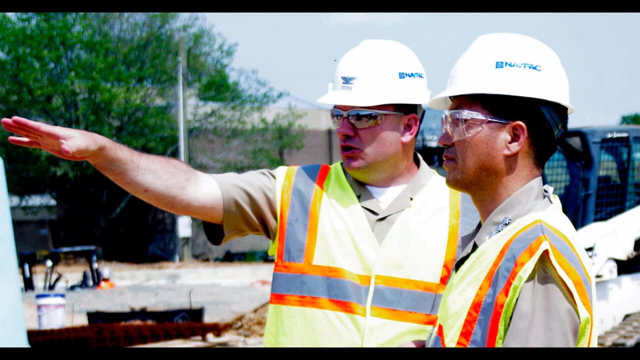 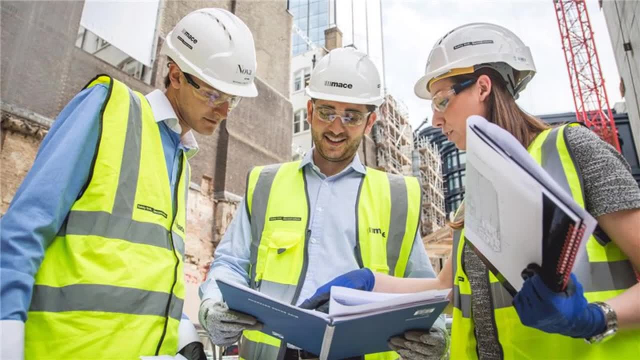 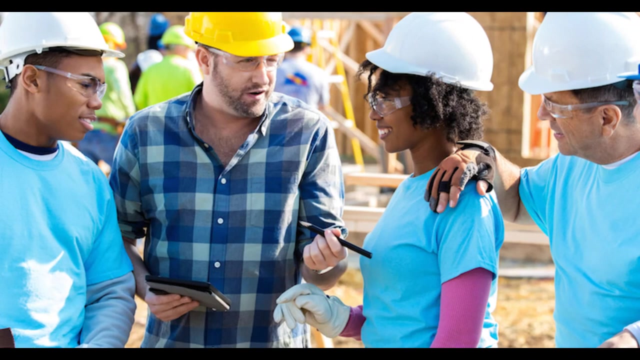 So they should encourage their engineering employees to become registered at the earliest possible date. They should encourage engineering employees to attend and present papers at professional and technical society meetings, or at least uphold the principle of mutually satisfying relationship between employers and employees with respect to in terms of employment, including. 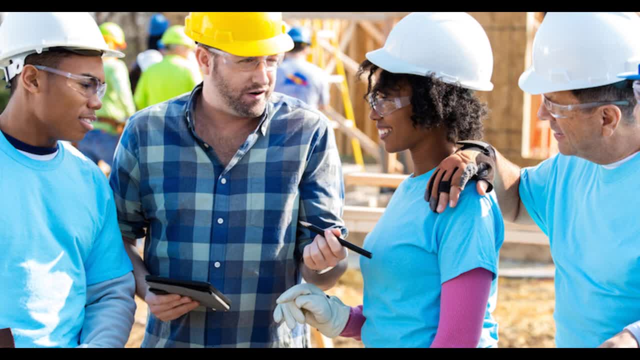 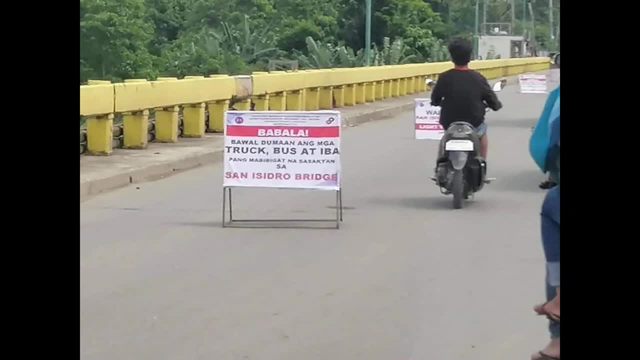 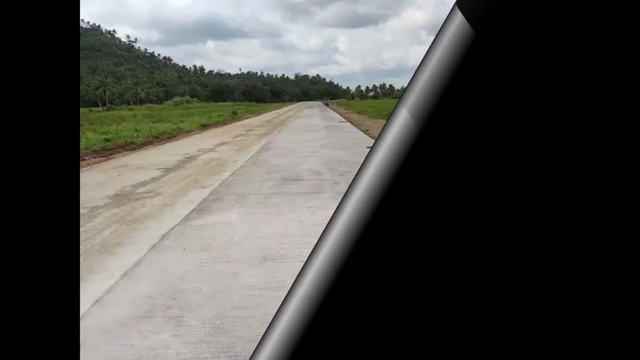 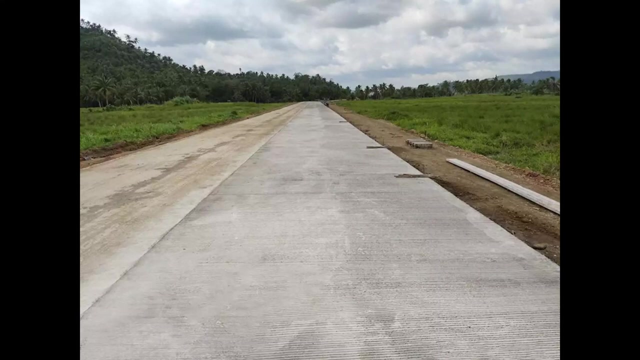 professional grade descriptions. This is the sample case that violated the fundamental principles and canons: The 9 Cebu City Barangay Road and Bridge Projects. At least nine southern Cebu City barangays were found to have used substandard materials in their infrastructure projects. 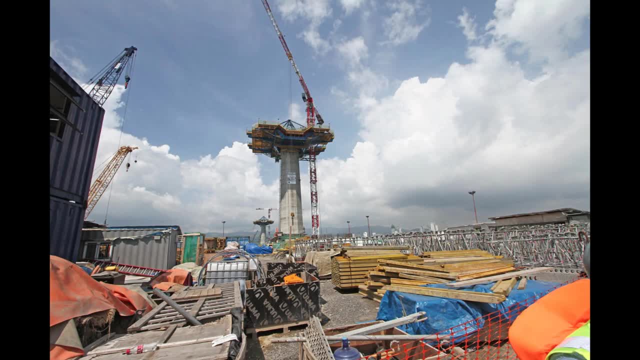 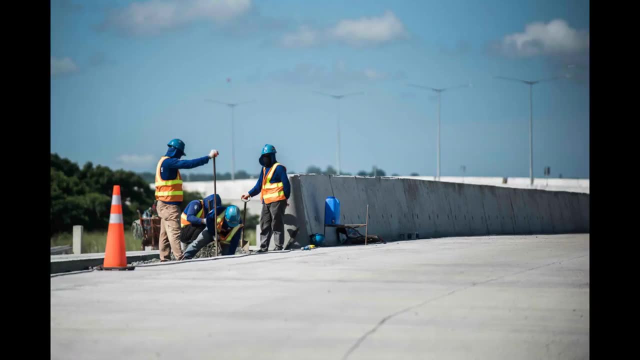 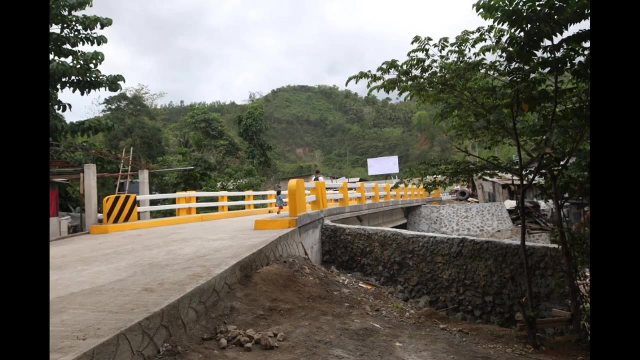 Engineers of the Department of Public and Highways Central Office were found to inspect the projects and to make the most appropriate corrections. The road projects lacked. asphalt salient, which caused the weakening of its joints. Mature and minor scaling were found in various parts of the road. 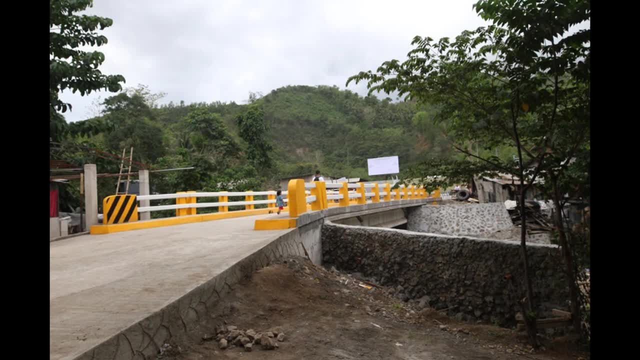 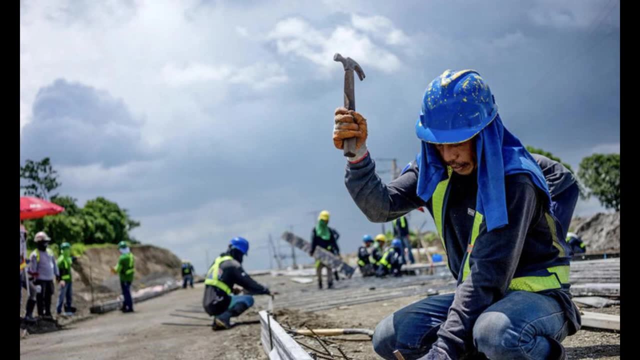 Poor workmanship. substandard boulders were found in the river embankment. Lack of supervision during the implementation of the project was evident. Some of the projects were substandard, raising suspicions that someone made money from the. someone made money from the project, So this is clearly a violation of fundamental principles. and canons.